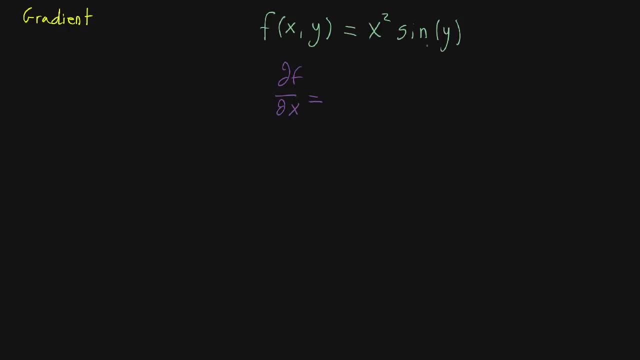 and y the gradient. So x is a constant. Well, in that case, sine of y is also a constant. you know, as far as x is concerned, The derivative of x is 2x. so we see that this will be 2x times that constant sine of y. 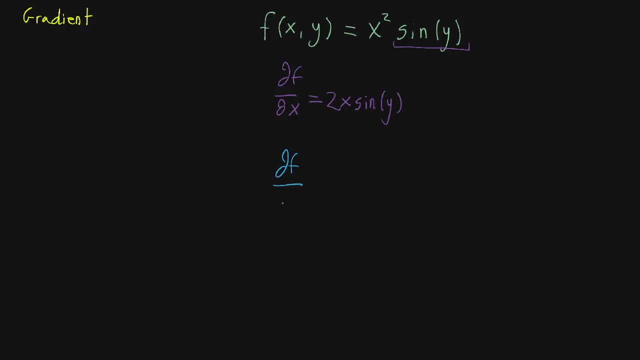 Whereas the partial derivative with respect to y. now we look up here and we say x is considered a constant, so x, squared is also considered a constant. So this is just a constant times sine of y. so that's going to equal that same constant times the cosine of y. 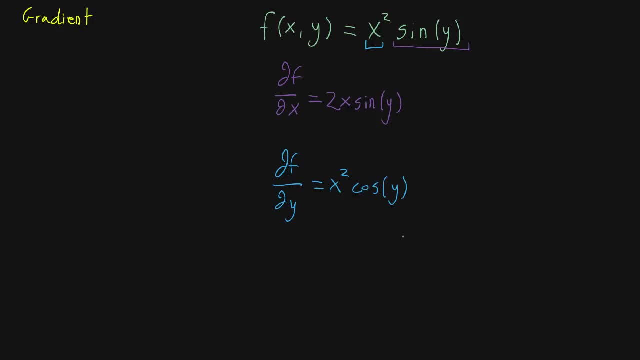 which is the derivative of sine. So now, what the gradient does is it just puts both of these together in a vector. And specifically- let me all change colors here- you denote it with a little upside-down triangle. The name of that symbol is nabla. 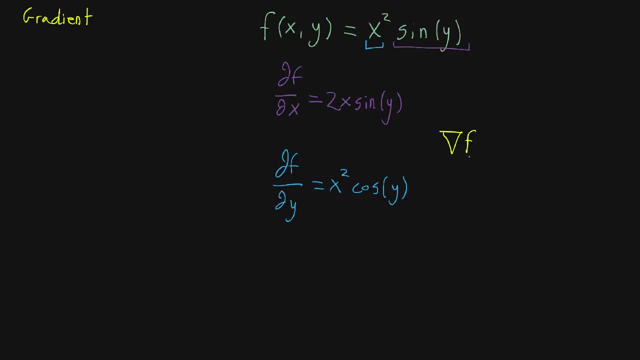 but you often just pronounce it del. You'd say del f or gradient of f, And what this equals is a vector that has those two partial derivatives in it. So the first one is the partial derivative with respect to x 2x times sine of y. 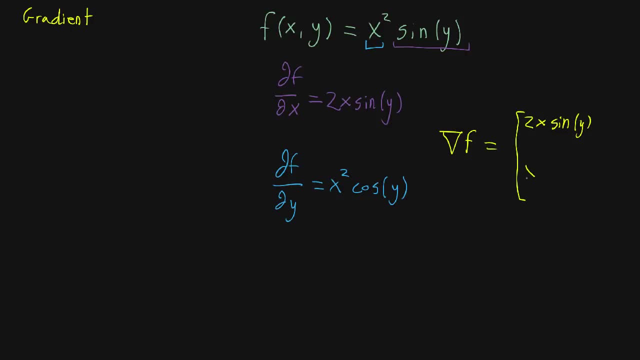 and the bottom one partial derivative with respect to y: x squared cosine of y. And notice, maybe I should emphasize: this is actually a vector-valued function, right? So maybe I'll give it a little bit more room here and emphasize that it's got an x and a y. 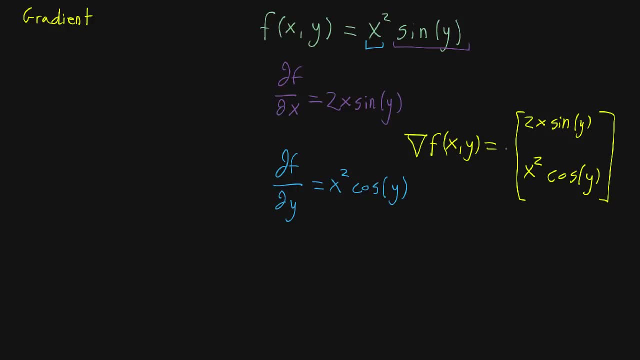 This is a function that takes in a point in two-dimensional space and outputs a two-dimensional vector. So you could also imagine doing this with three different variables. then you would have three partial derivatives and a three-dimensional output And the way you might write this more generally. 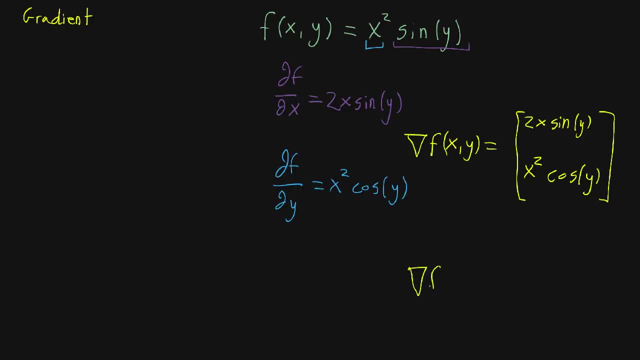 is. we could go down here and say: the gradient of any function is equal to a vector with its partial derivatives, Partial of f with respect to x and partial of f with respect to y, And in some sense, you know, we call these partial derivatives. 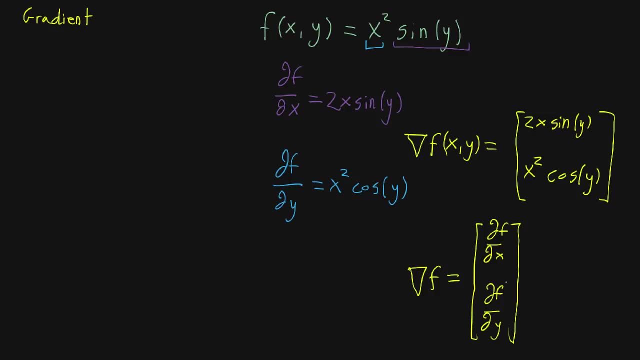 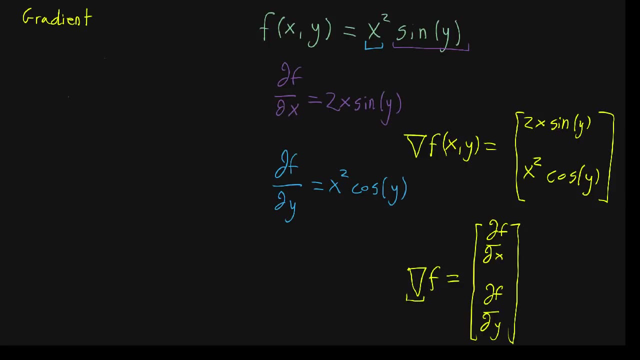 I like to think of the gradient as the full derivative because it kind of captures all of the information that you need. So a very helpful mnemonic device with the gradient is to think about this triangle, this nabla symbol, as being a vector full of partial derivative operators. 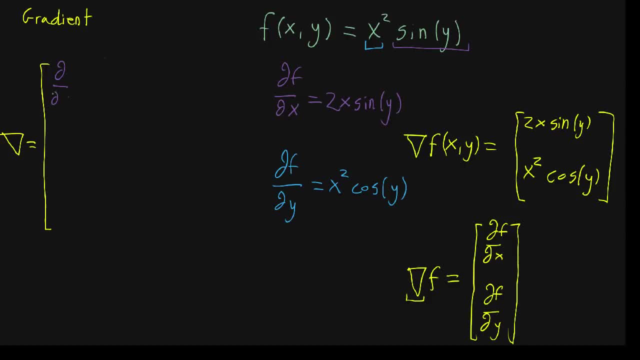 And by operator I just mean, you know here let's like partial with respect to x, something where you could give it a function and it gives you another function. So you give this guy, you know, the function f. 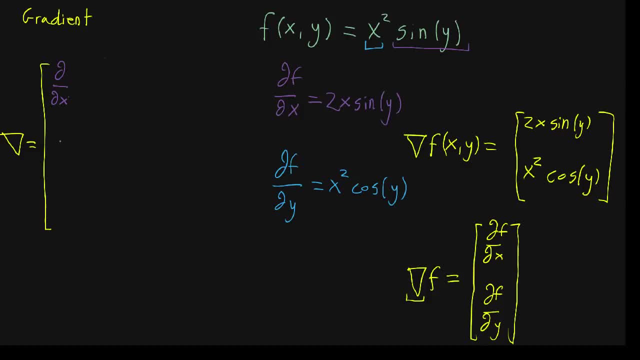 and it gives you this expression, this multivariable function, as a result. So the nabla symbol is this vector full of different partial derivative operators, and in this case it might just be two of them, And this is kind of a weird thing, right? 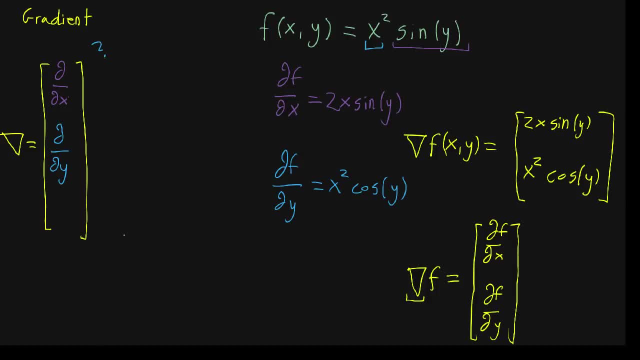 Because it's like: this is a vector. it's got like operators in it. that's not what I thought vectors do, But you can kind of see where it's going and it's really just a. you could think of it as a memory trick. 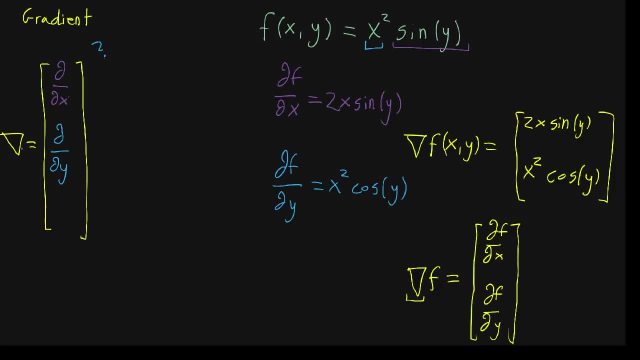 but it's in some sense a little bit deeper than that And really, when you take this triangle and you say, okay, let's take this triangle, and you can kind of imagine multiplying it by f, really it's like an operator taking in this function. 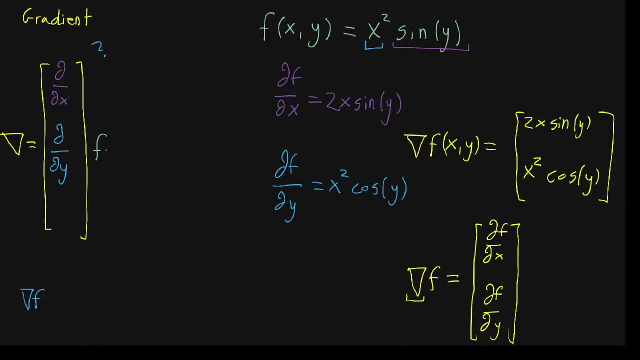 and it's going to give you another function. It's like you take this triangle and you put an f in front of it and you can imagine like this part gets multiplied- quote unquote- multiplied with f. this part gets, quote: unquote- multiplied with f. 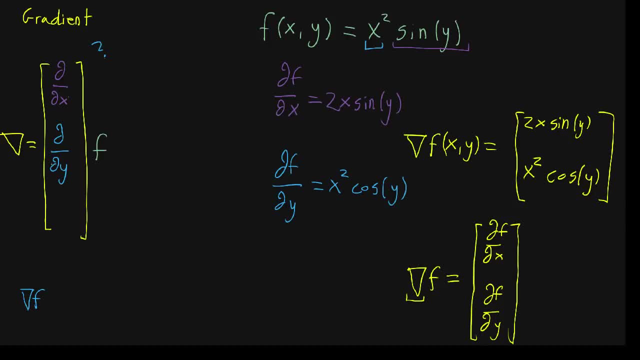 but really you're just saying you take the partial derivative with respect to x, and then with y, and on and on. And the reason for doing this? this symbol comes up a lot in other contexts. There are two other operators that you're going to learn about. 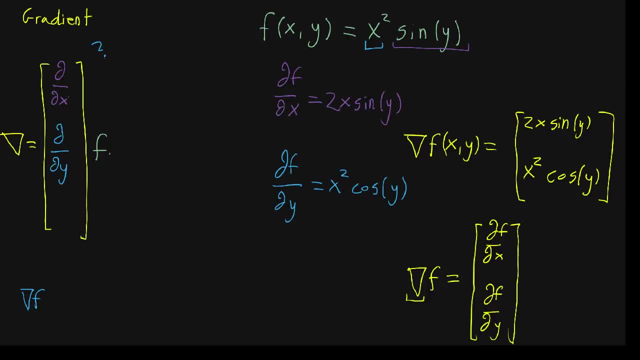 called the divergence and the curl. We'll get to those later, all in due time. But it's useful to think about this vector-ish thing of partial derivatives, And I mean one weird thing about it. you could say, okay, so this nabla symbol. 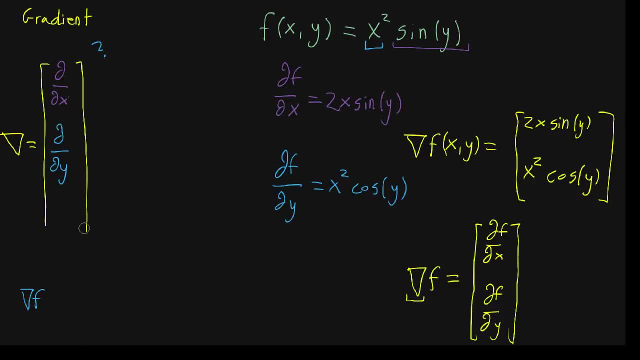 is a vector of partial derivative operators. what's its dimension? And it's like: how many dimensions do you got? Because if you had a three-dimensional function, that would mean that you should treat this like it's got three different operators as part of it. 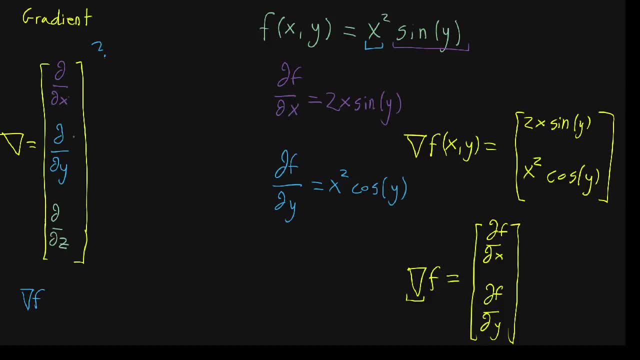 And you know, I'd kind of finish this off down here, And if you had something that was a hundred dimensional, it would have a hundred different operators in it, And that's fine. it's really just again kind of a memory trick.